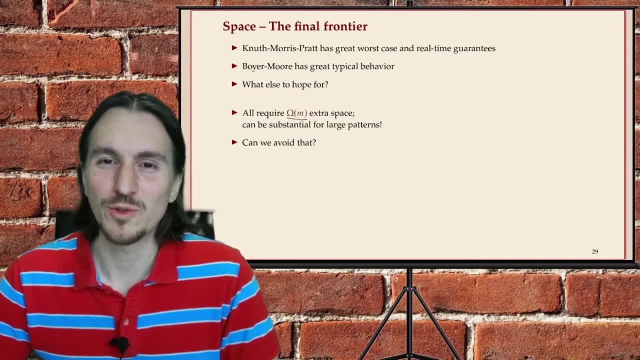 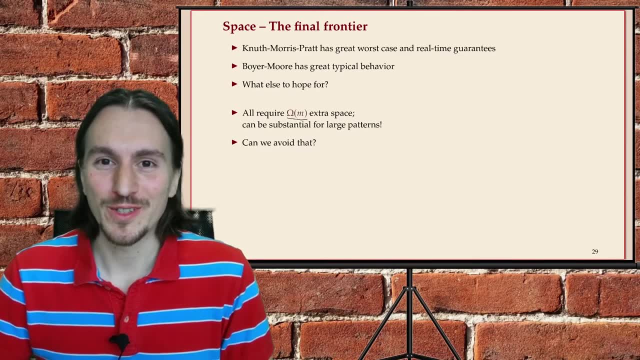 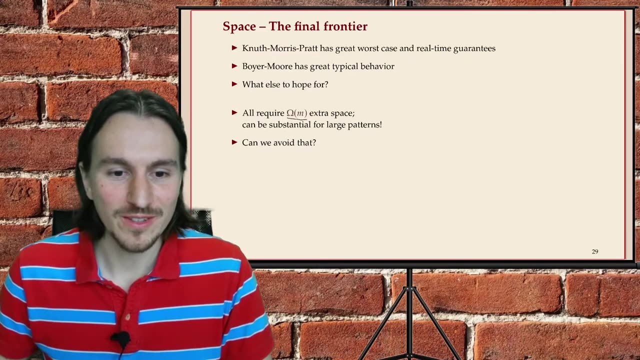 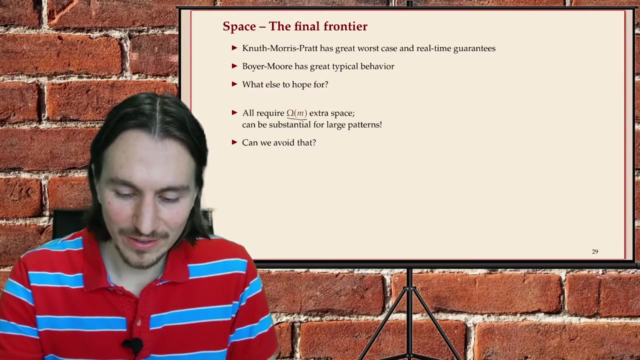 It's usually not such a big deal because you have to store the pattern itself, but it's space on top of that And it's also a nice theoretical question if we can avoid that or if that is inevitable. And yeah, as it turns out, this is very much avoidable, And so the idea for that is from: 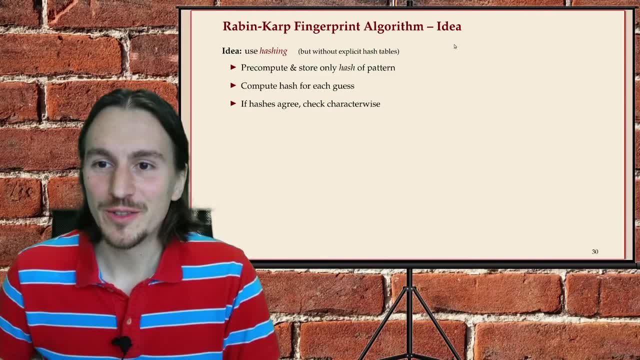 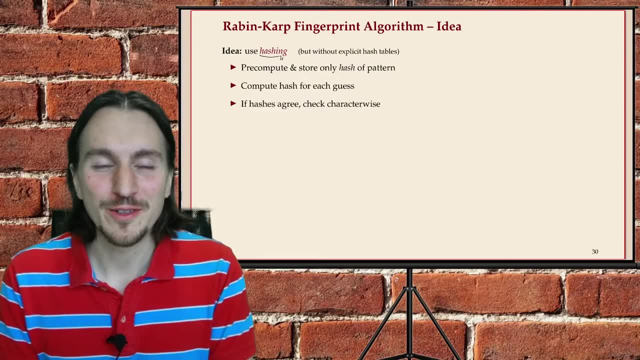 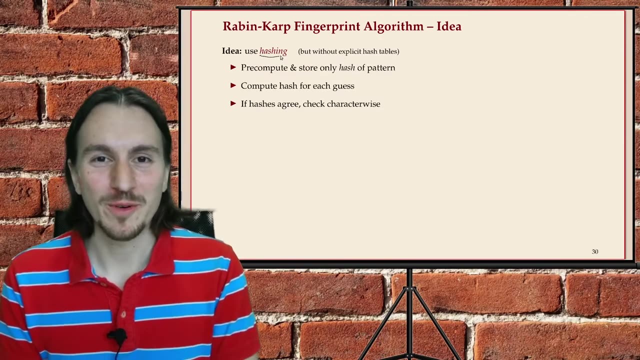 a very different field. We use fingerprinting. It's otherwise known as hashing, And if you've done an undergraduate Yeah, algorithms class, data structures class, you will definitely know about hashing. I'd love to talk more about it. Maybe it should be part of unit two, but it was already quite 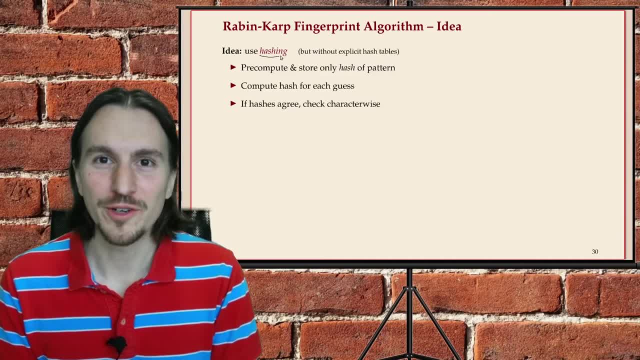 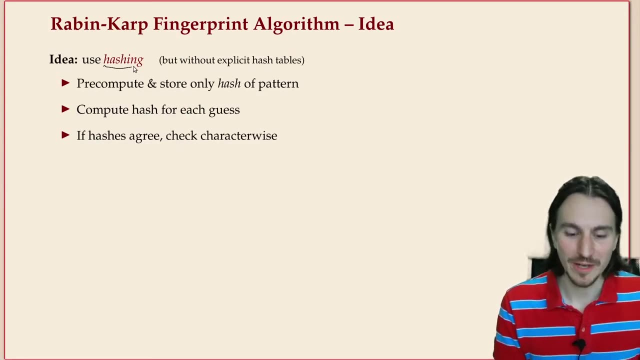 full Hashing is another way to realize unordered dictionaries, And for that it's usually the choice in practice because it has just great average case behavior. Here we just use the main idea of hashing and do it in a slightly different way. What? 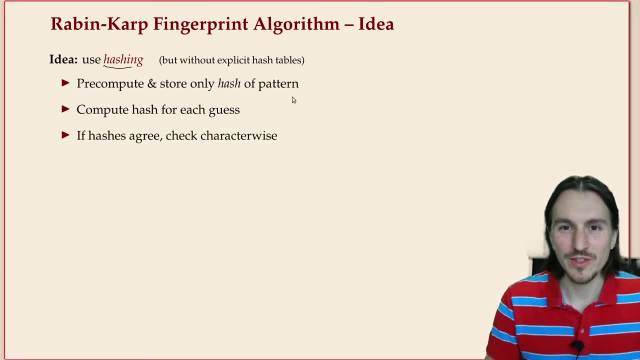 we do is We compute a hash of the pattern. So instead of this long string- that could be hundreds and thousands of characters- we compute a small number, relatively small number, maybe one int, that represents this pattern. That won't be without some loss of information. 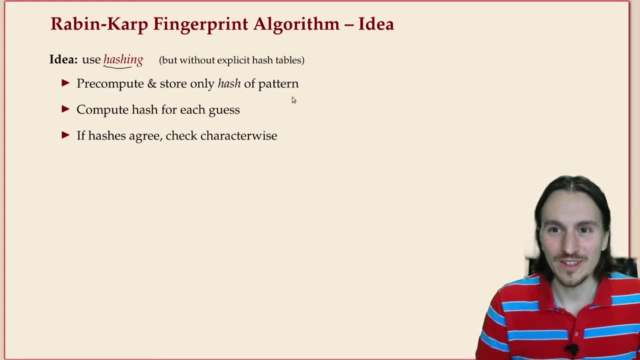 but still it will be good enough in a well-defined sense. Then we also compute for each guess, So each potential position in the text. we compute a hash, And if the hashes agree there might be a match. So then we check character-wise if 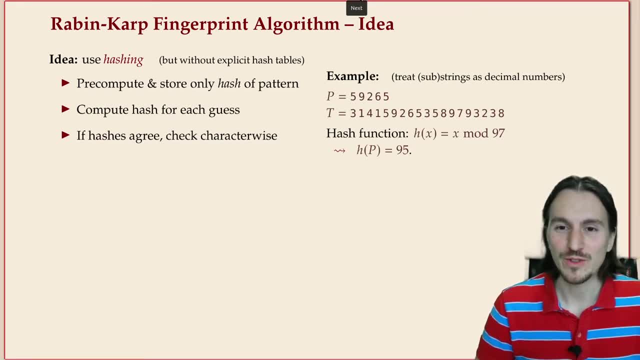 this is really a match. There could be false positives in that. the hashes match, but the strings are different. That's because it's just a fingerprint and that's not an identical representation of the entire thing. Maybe fingerprint is a bit of an unlucky name, because 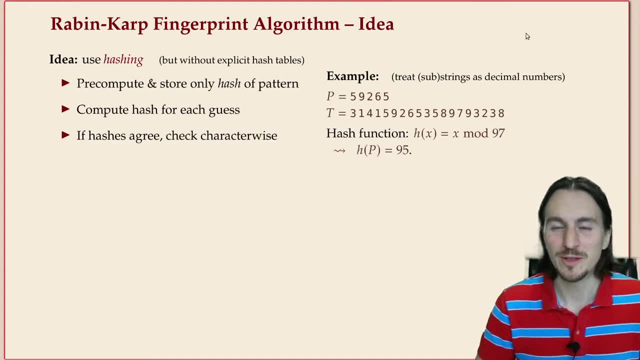 people think of fingerprints to be unique for each human, Whereas here Hashing really is not unique. There are different patterns that hash to the same fingerprint, So let's do an example here where to make the presentation a bit nicer. I'm assuming. 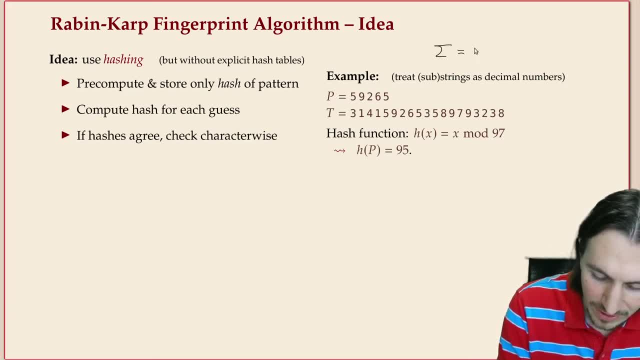 that the alphabet is just the decimal digits. There's not really any meaning to the numbers. So these are just characters and we interpret them for the hash function. But that is only by convention And you can do this with any other characters And you. 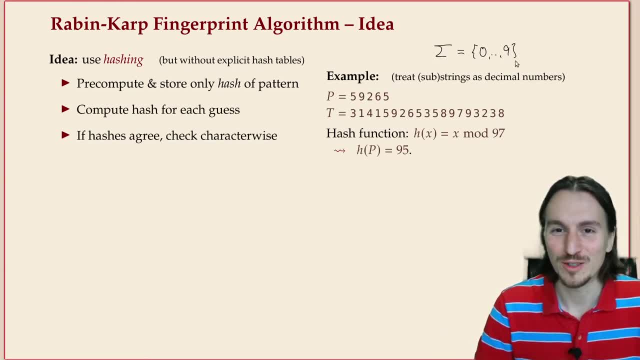 can do this also by not following the usual convention of what these digits mean. You can reverse the order or do whatever you want. So here's a pattern. Here's the text. This is also nice, because it makes it a little tougher for humans to spot the pattern in the text. But if you look closely you'll. 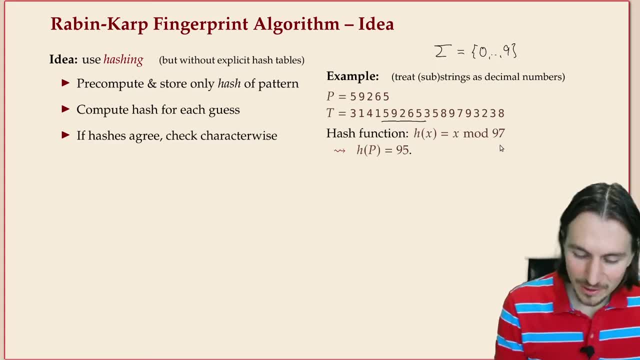 see, there is actually an occurrence here, And we'll use as a hash function Five digits interpreted as a decimal number, and then take that number modulo 97. Why 97? Because it's a prime number and it works reasonably well to use such a number. 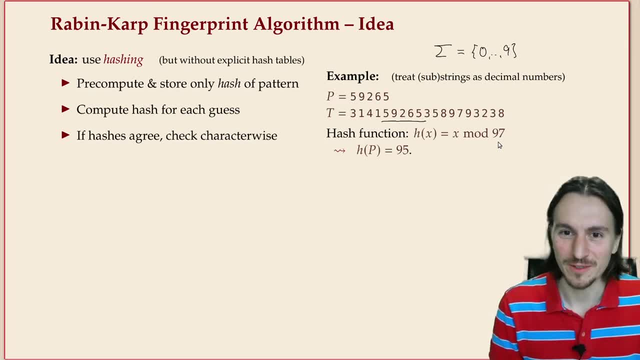 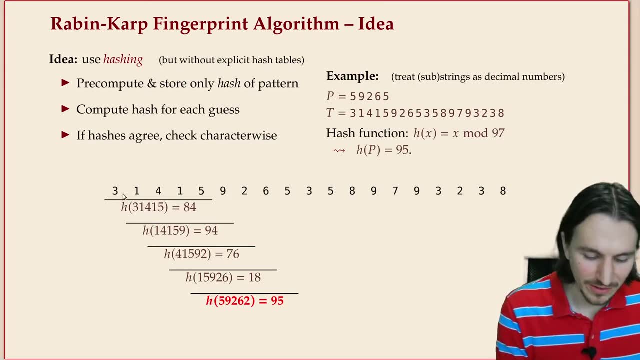 That's the only reason, And usually you choose something like this at random. So here's our text. The conceptual idea of Rabin-Karp is to compute the hash value of five consecutive digits. This one is not 95, which is the hash of the pattern. 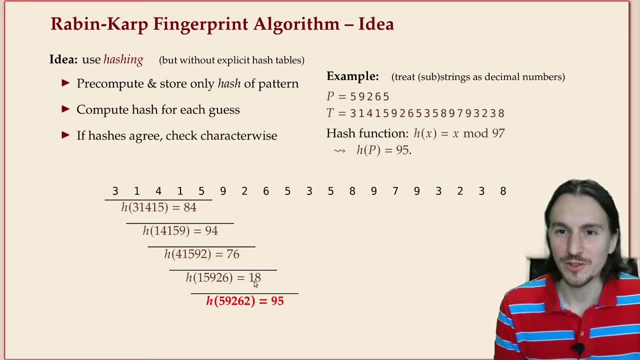 If you keep going, you find all of these can be excluded by just looking at the hash, because the hashes already don't match. Then the part of the text and the pattern cannot be the same. But if you start here, 59265,, that actually is the pattern and it has the same hash. 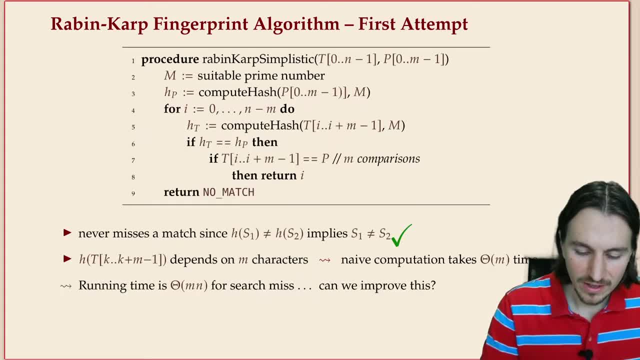 So you found an occurrence here. Very simple idea, Very easy to put into code. If you've seen hashing before, you might not be surprised that you want to start with a suitable prime number of a certain range. I don't want to go into detail with this. 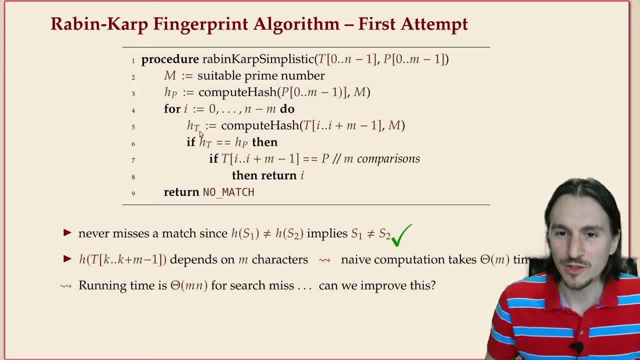 We compute the hash of the pattern and then, for every possible position in the text, we compute the hash of the portion in the text, And if the two match, Then We still have to do the character wise comparison. As I told you, the hash could be the same even though they are different. 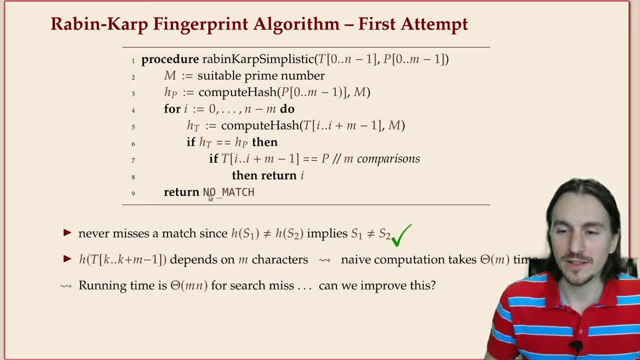 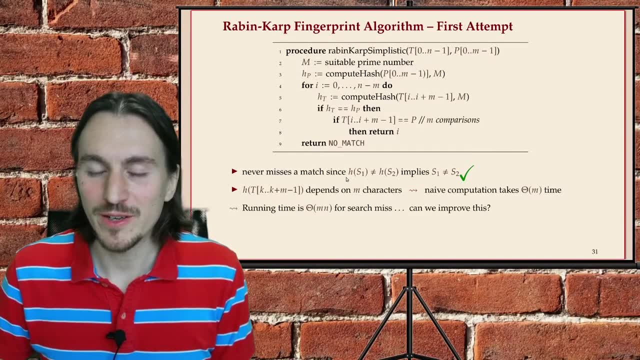 But then we return the match if we actually found it, And if not, we return that there is no match. Now, this is fine. It never misses a match, since if the hashes are different, the text is different. That's the core property of a hash function. 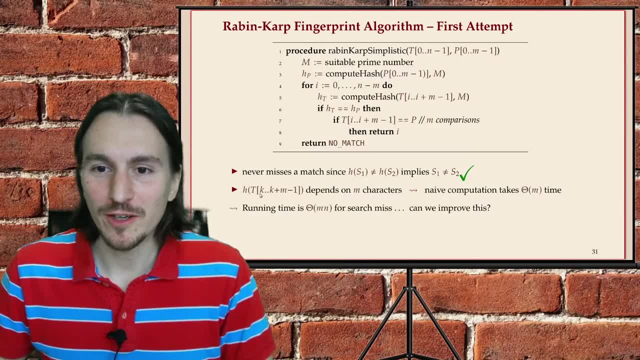 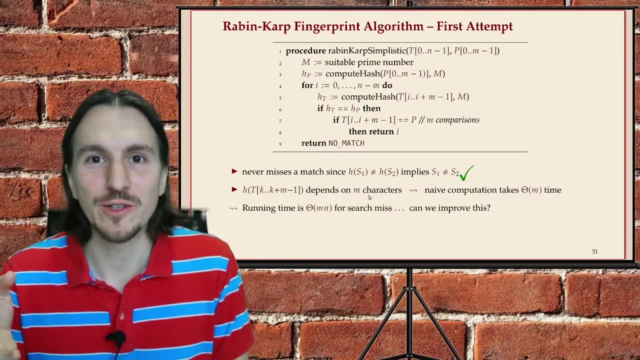 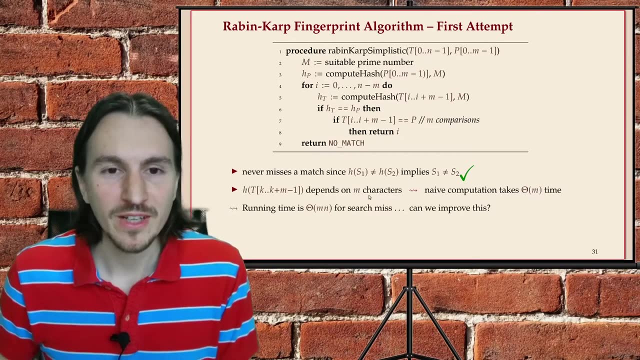 The hash value that we compute, In particular The portion of the text. It depends on the m characters in the text. That was the idea. The hash function we use was just interpret this part as a number and then take that number and modulo a prime. 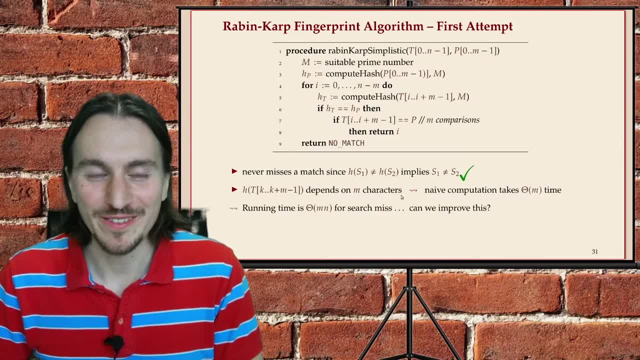 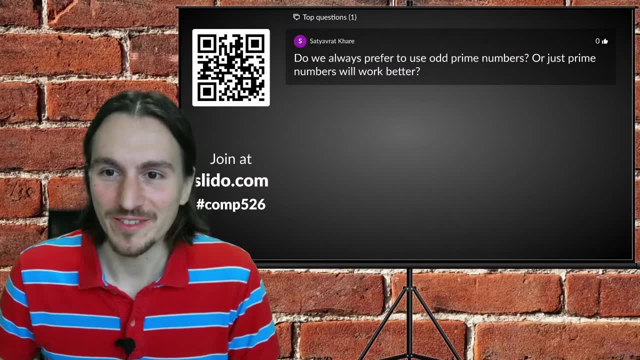 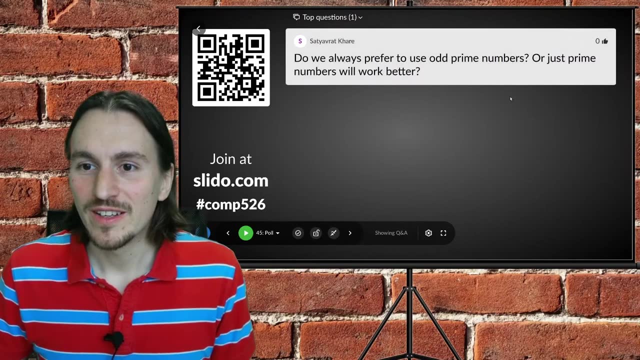 Yeah, I was about to answer the question. I've seen your question on Slido, So maybe this is a good point to address that part Just very briefly. Yes, We kind of Prefer prime numbers. Well, there's not so many even prime numbers. 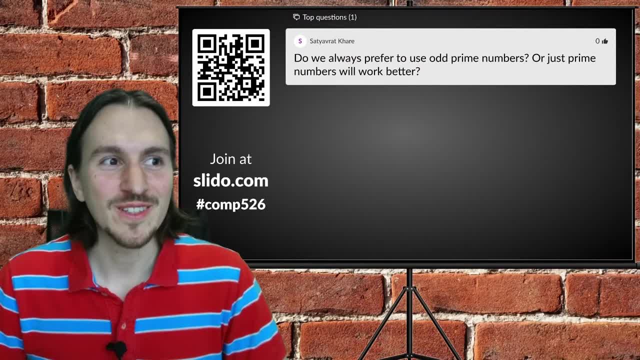 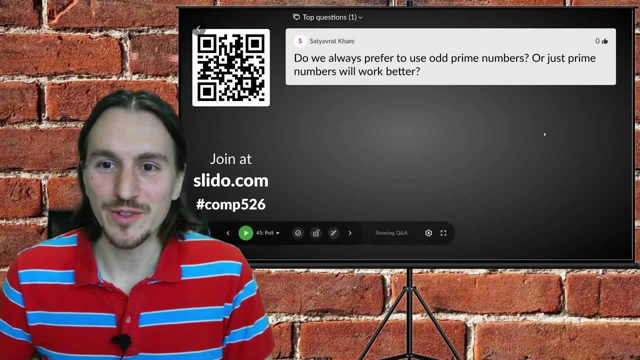 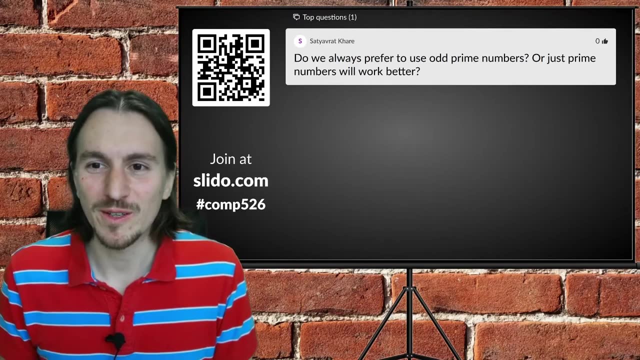 There's only one and that's too small. So what you really want is a prime number that has roughly the right size, And the size of the prime number gives you controls- the probability of hash collisions. So you want this to be as big as you can make it without taking a performance hit. So maybe a prime number close to the size, The largest integer you can represent, is probably a good choice. So yeah, we want prime numbers because then collisions are much less likely. For more details on this you would have to study hashing in more detail, and that's maybe. 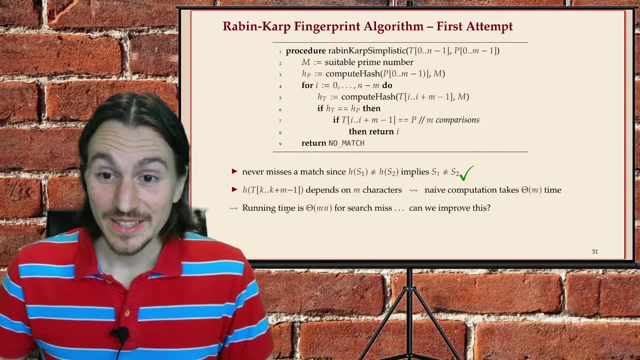 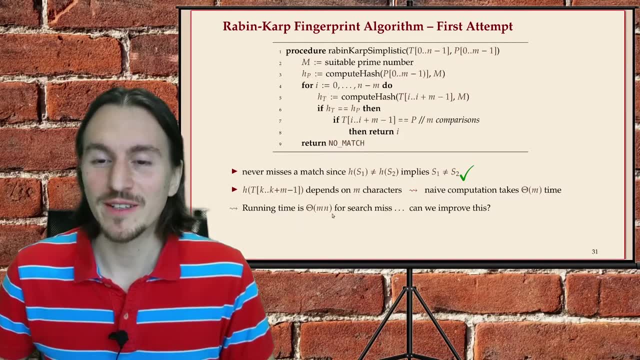 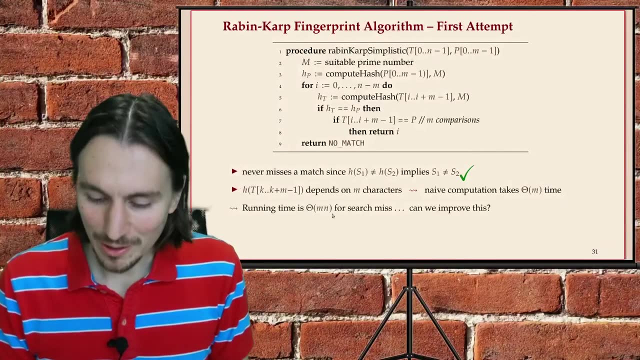 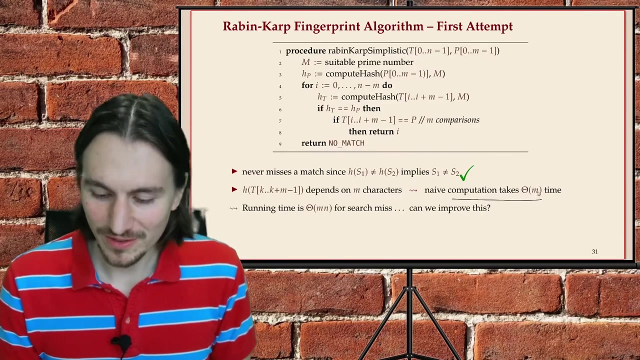 for another time. Now, the worst case, running time, and actually the running time on any input for this code is still n times, And the reason for that is that we have to compute the, we have to compute the hash value for each position in the text and we do this n minus n times and it takes n time each. 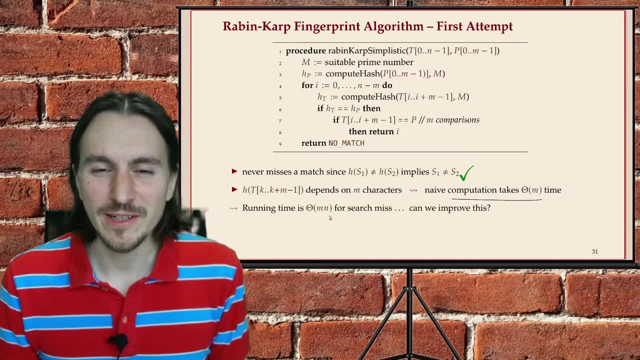 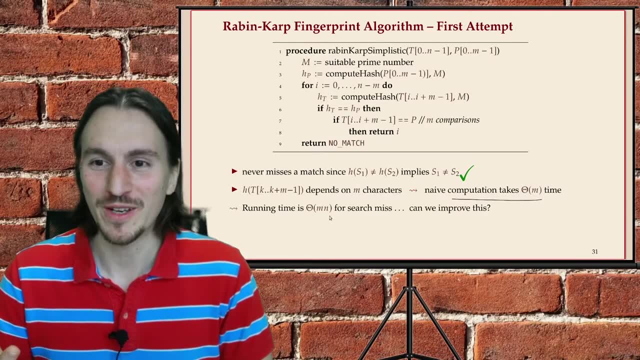 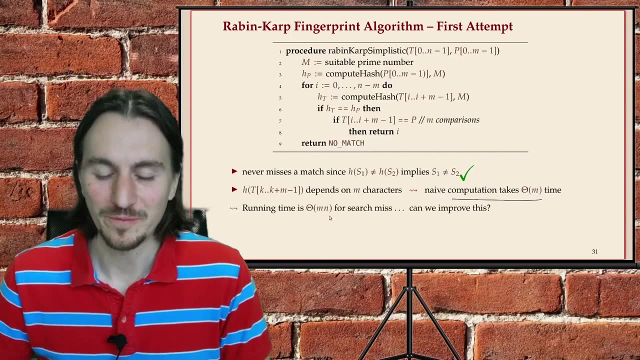 So that's n times m. So it looks like our great idea with the fingerprinting wasn't really worthwhile doing it, because to just compute the fingerprint we already spent as much time As we spent previously To find to check if that is there is an occurrence of the pattern at this point. 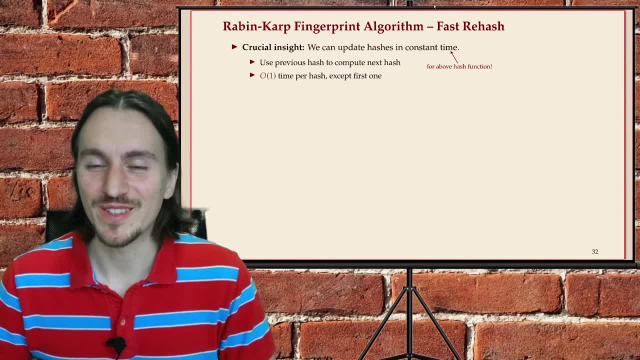 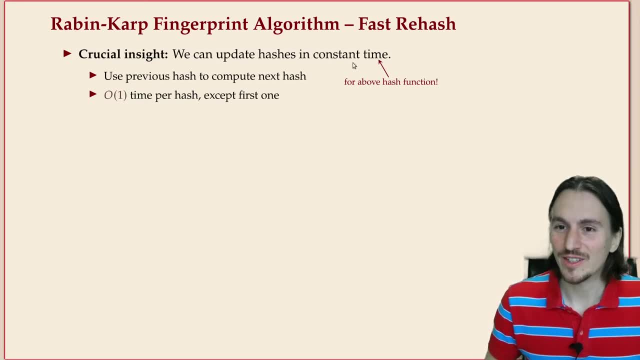 So that's too bad, But fortunately we can fix this. The main insight of of Rabin and Karp is that we can update hashes in constant time if we move from position i to position i plus one, And that only works for specific hash functions, exactly the one that I've had above interpret. 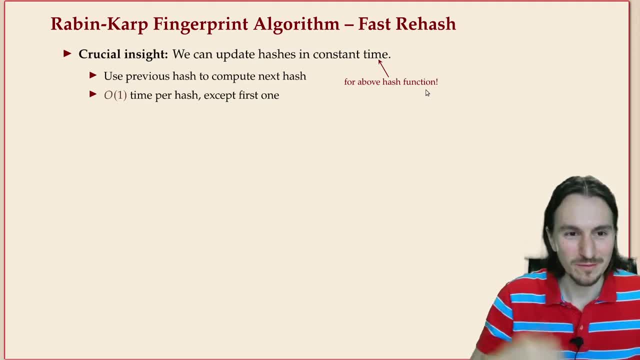 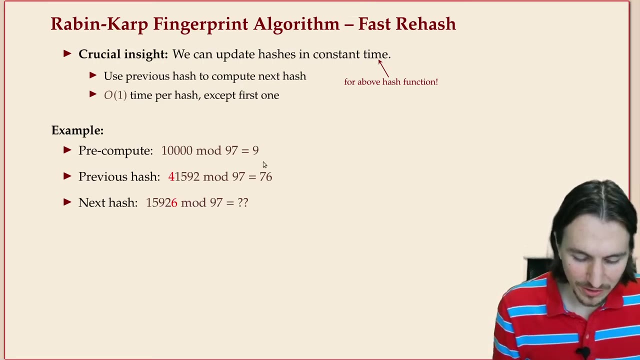 things as a decimal number Or as a number with radix size of your alphabet, and take it module or something. Let me briefly sketch how this works. This is sometimes called a rolling hash. We do some pre computations, Basically the well, the largest possible value plus one. 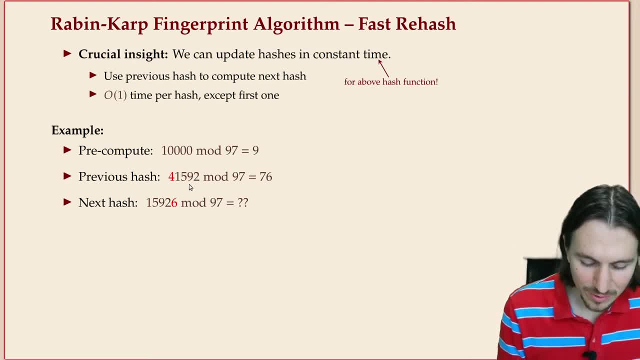 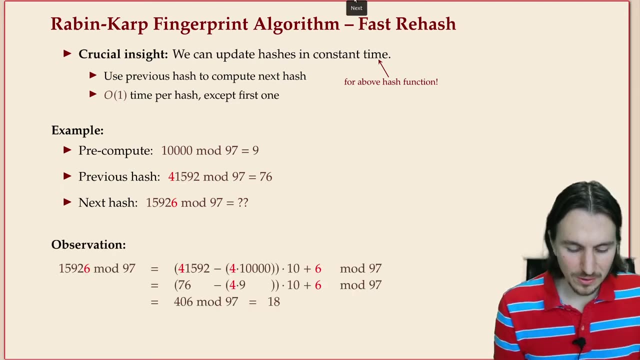 Um, Then We take the previous hash And we would like to find the next hash. So notice that these four characters are the same. They're just shifted over by one position and you append a new one. Now, if you look into what the new hash value is, 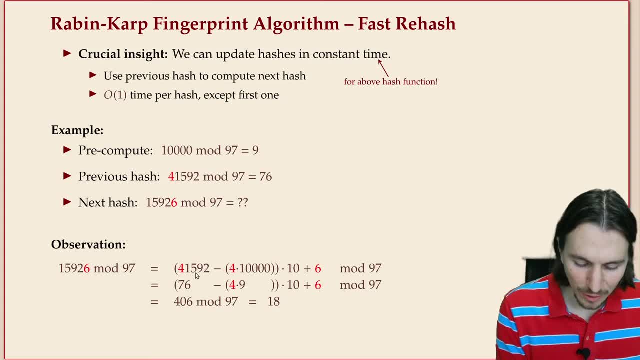 The new number this: this number is the old number subtracted four times Was that ten thousand? That's because you want to get rid of the first digit. That subtraction would leave you with a thousand five hundred ninety two. Then you multiply by ten to shift the number one over and you add the new digit. 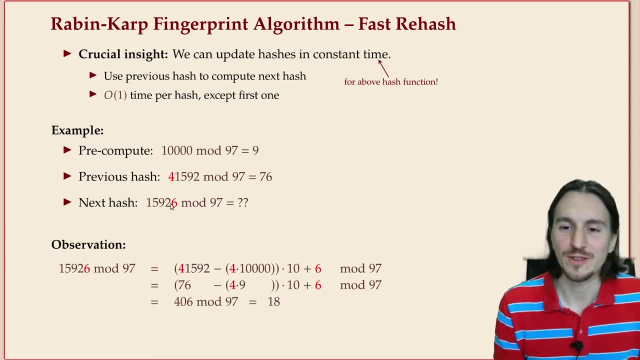 That is how you get from this number in decimal to this number in decimal, And while taking modulo doesn't make a difference. here it's it's the same number, So you might as well do this. The trick now is if you compute in modulo, 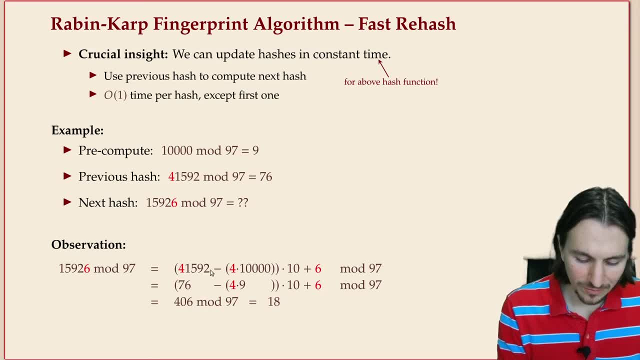 You can compute, You can compute modulo before you do the arithmetic operations, and that's again something where it's important. you're operating with a prime And so you can compute this modulo ninety seven first, but that's the old hash, so we already know this. 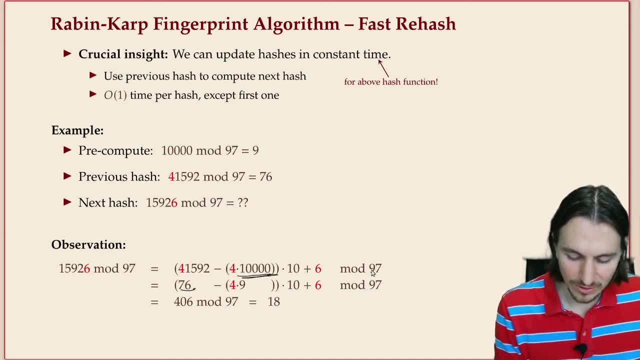 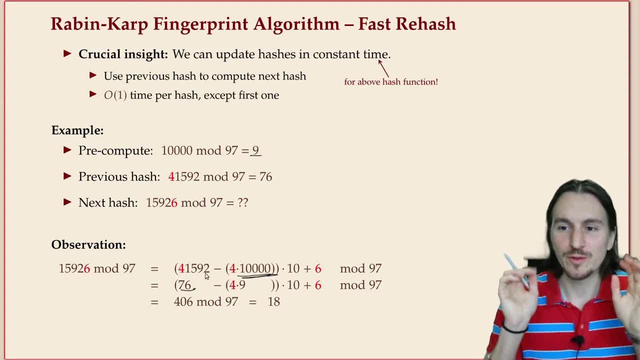 That's the old hash, That's the point. These the pattern itself or the portion of the text that can be very, very large. It depends on the size of the pattern you're given. But modulo, that prime, that's something you have under your control. 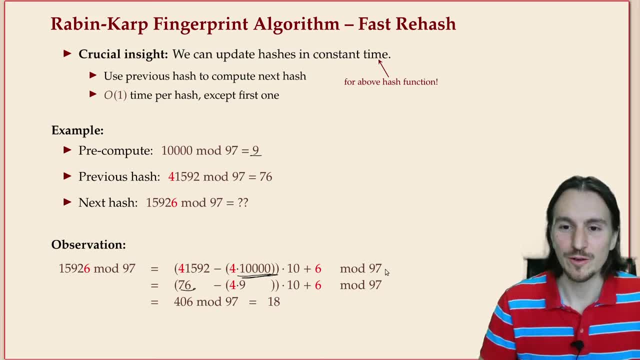 You can choose the prime small enough so that the numbers are small enough for you to compute in constant time, And so you can just do this computation instead of working with these humongous numbers, and do one more modulo step, and then you have the new hash. 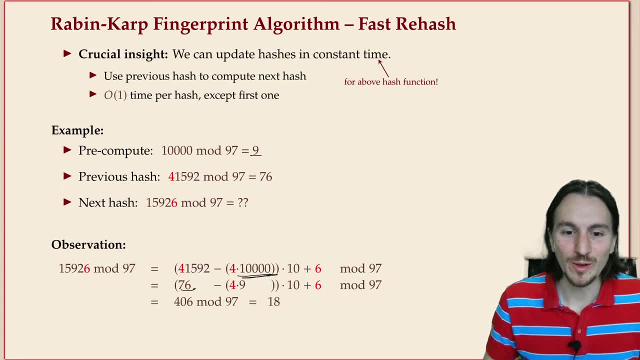 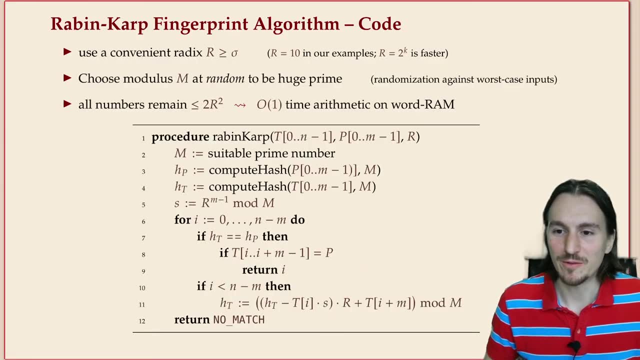 All right. right, That's a neat way to exploit this specific form of the hash function, And doing that in code gives you the Rabin-Karp algorithm. So a few more comments. You pick some radix. Well, it has to be bigger than the size of the alphabet. It was 10 in our examples. 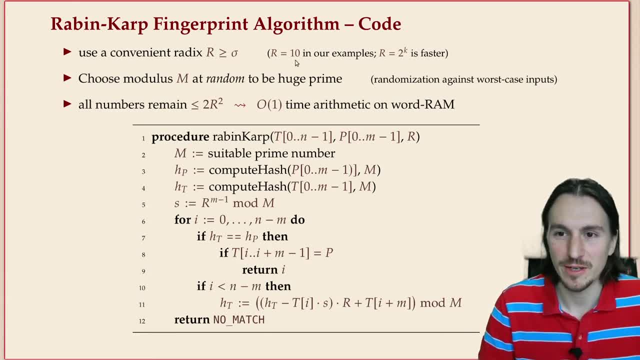 Then we just had the usual decimal numbers, but anything really works. A power of two is convenient. Then you can do the shifting with bitwise shifts. but that's minor optimizations that need not concern you for this class. And you choose a huge prime number. that's random. 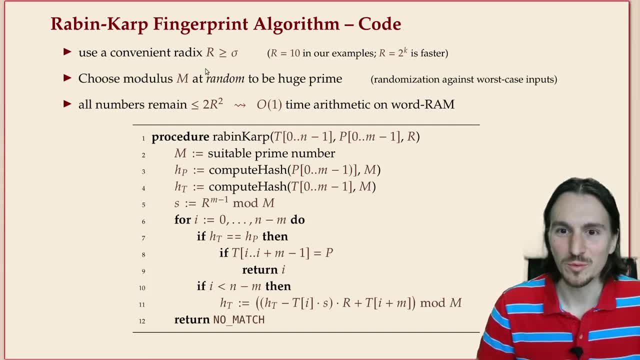 but not too big, so that you can still work with these numbers efficiently. And all numbers that you work with then remain bounded in terms of the radix. So in our case, if r was 10, we have numbers of at most size 200. And you can choose r so that it matches up with the word size. 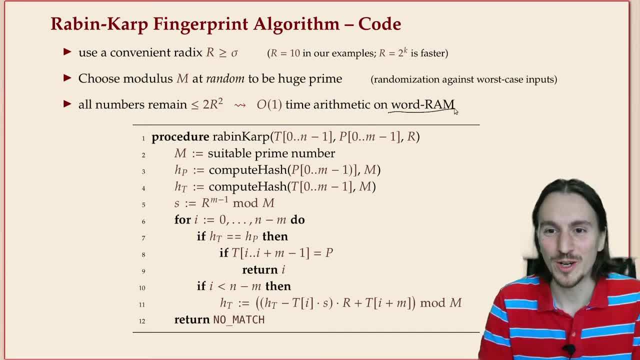 of your word RAM, Remember. our machine model assumes that you can do arithmetic operations in constant time if the numbers are not too big, And so you can do this update in constant time. How does that look in the code? Not too complicated, actually. The only change is if you 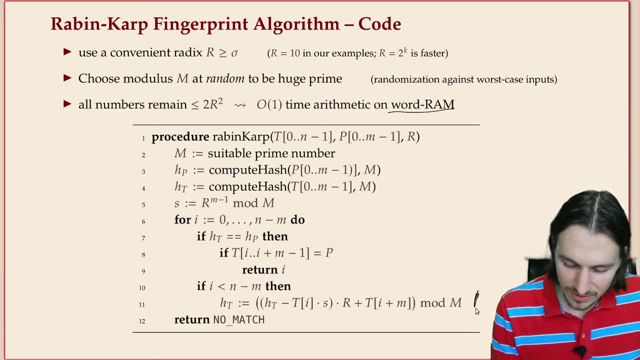 update the hash here. That's the only real change from the previous slide. You do exactly that computation that we had. You subtract the first digit, shift it by the radix and add the new digit and do one computation with the modulo, the prime, That's Rabin-Karp string matching with the rolling hash. 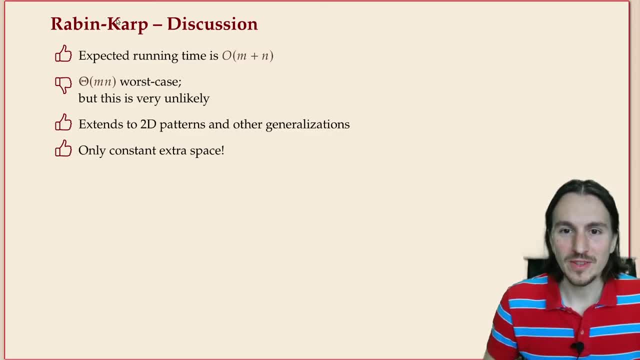 How well does this work? The worst case is still n times m, which sounds maybe disappointing, But this only comes from the fact that in a very, very unfortunate situation, you might have to always do the slow check If you find, for some reason, a text where you always have. 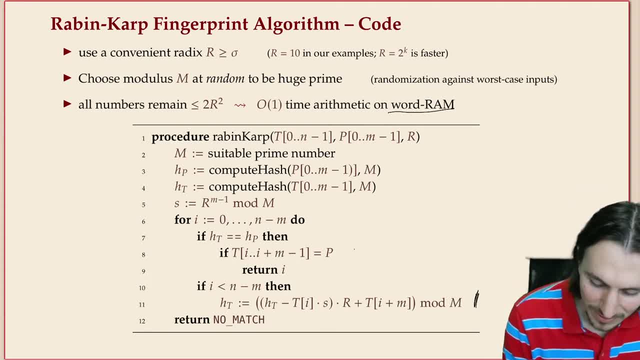 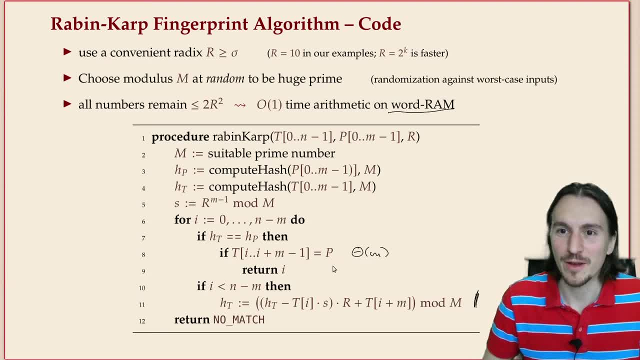 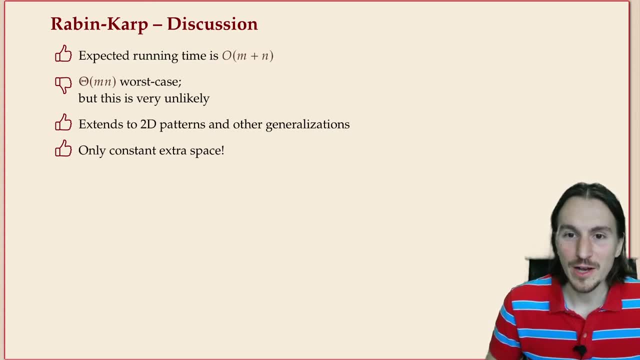 that needs theta m time, And if you have this for every possible guess, then you will need n times m. but this is very unlikely if you have a non-maliciously chosen texted pattern And in particular, if you're looking just for the first occurrence. 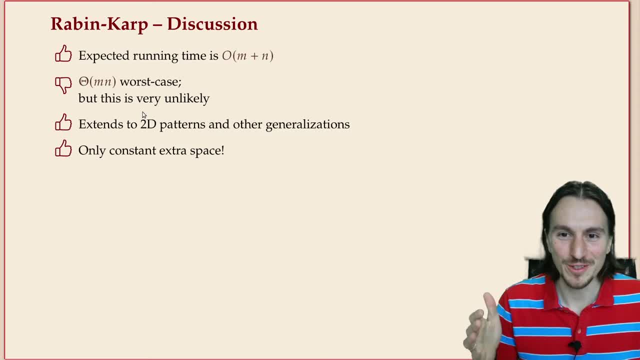 it's astronomically unlikely. You will never see this really happen in practice. It's probably more likely that your computer is dying from some solar flare or whatever, And the expected running time indeed is optimal, linear in the text length and the pattern length. 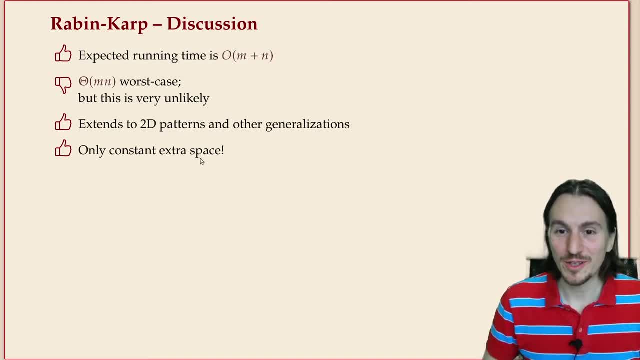 And it has some other nice features. First of all, it only needs constant extra space. We're only storing the fingerprints and not some pre-computed other information about the pattern. And secondly, this algorithm, unlike all the previous ones, is easier to generalize to other scenarios, For example to 2D patterns, which, in other words, 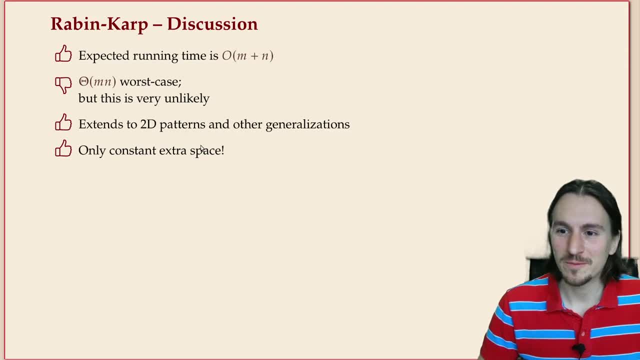 are images. pixel images are not far from a two-dimensional text, where you have rows and columns and a symbol in each position, So you can use Rabin-Karp-style algorithms to also find patterns in 2D or higher dimensions, And this is something where the other algorithms 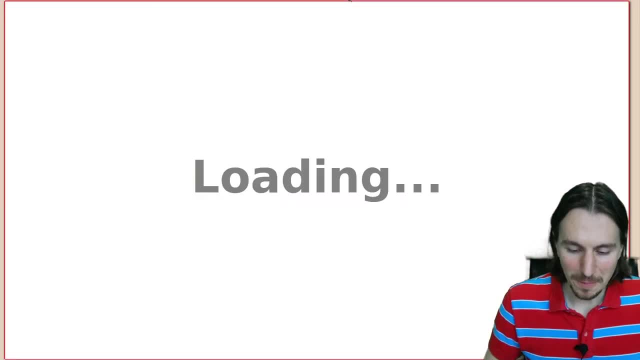 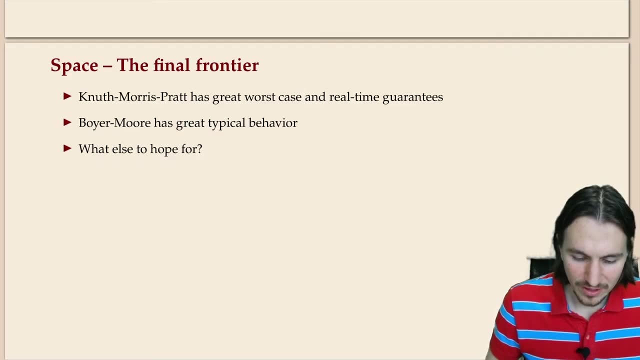 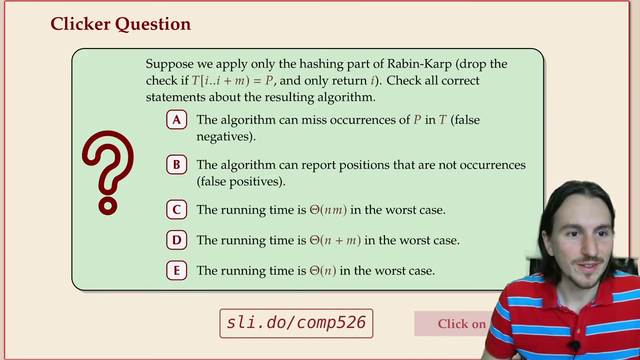 seem to generalize. well, Okay, that was not what I wanted. I have another question for you to see if you're following along. That's what we've seen, So similar to the previous question. a little test if you follow this beyond the superficial statements I made. 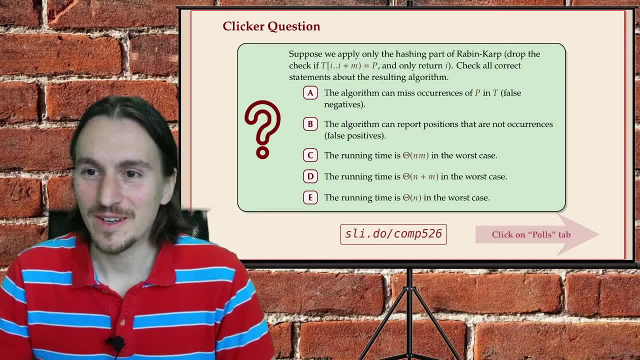 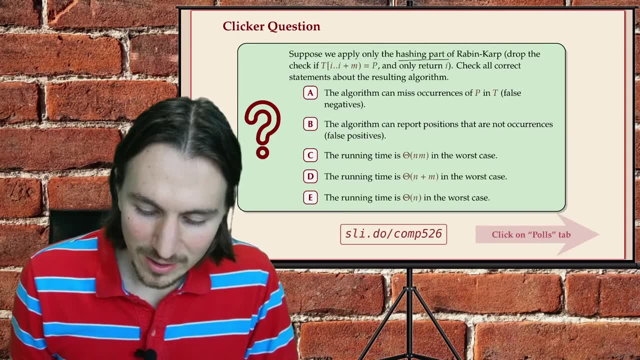 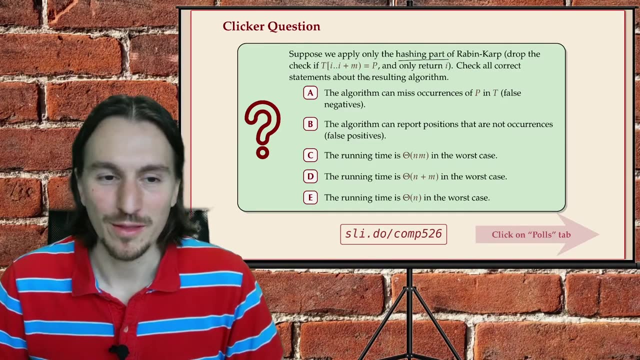 So give the question a careful read. It says we're only applying the hashing part of Rabin-Karp, but we skip the check. And what can be said about the method? And again, several of the answers are correct, so check all of them. 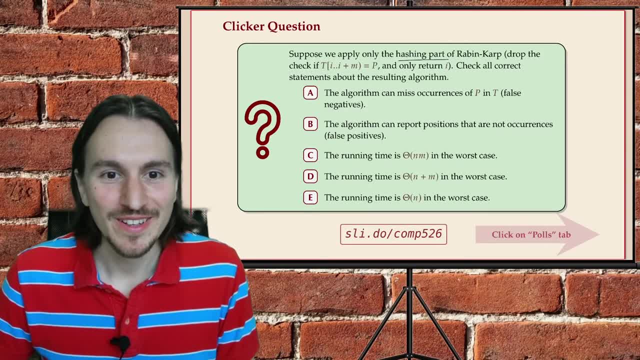 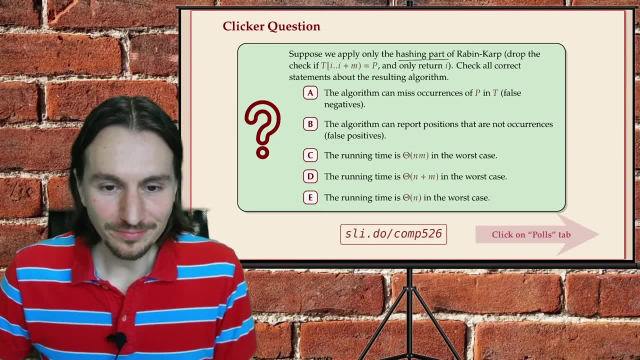 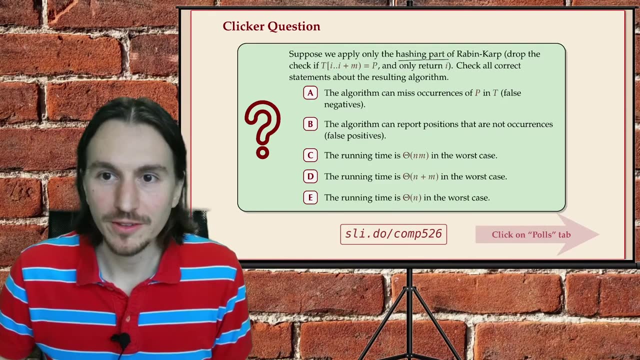 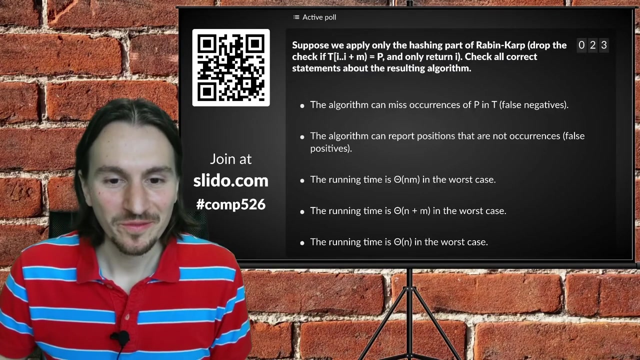 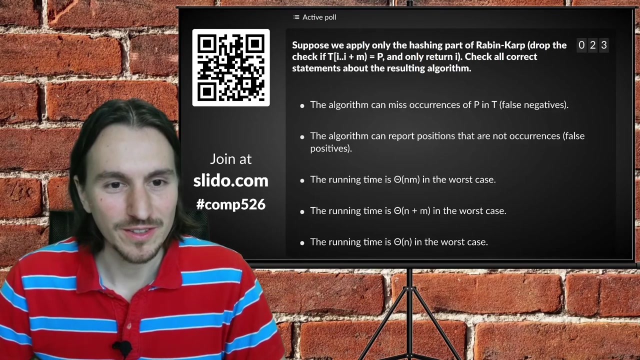 And I'm waiting for the usual 25 people. at least We're at 20, 22.. Maybe for this one I'll give you another minute to think about your answers, because this is needs a little thought to digest all the different possibilities. 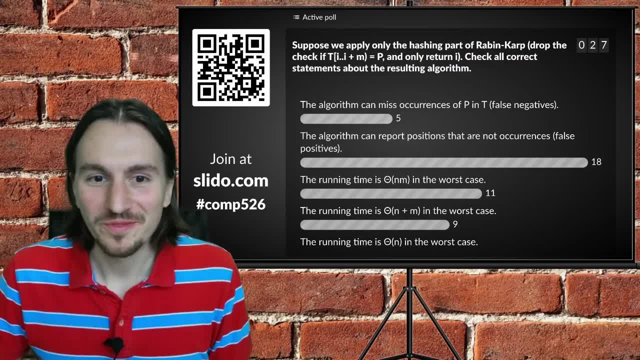 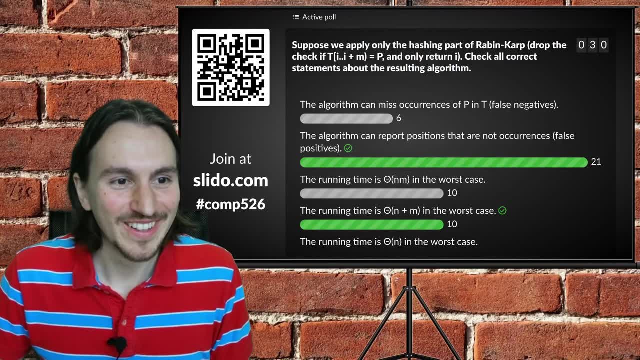 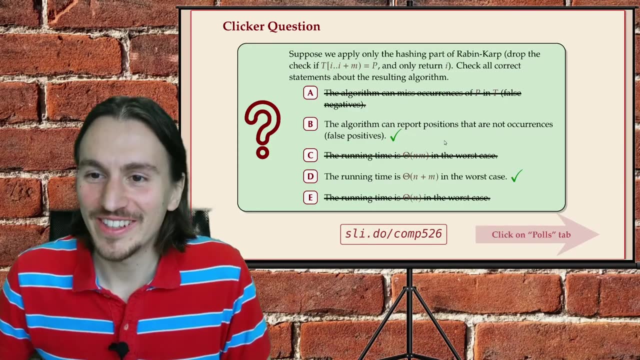 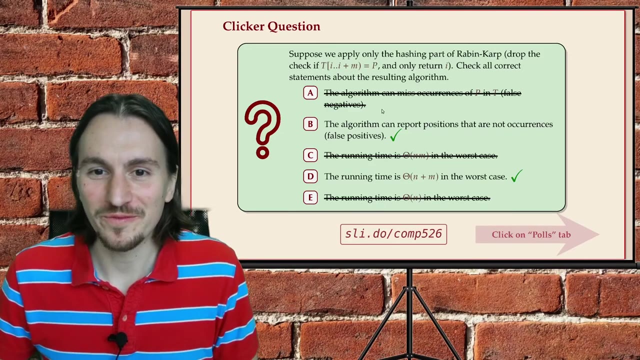 All right, There we go. Most of you figured this out, but I caught you with one of the others. I'll lock your answers in now, Okay, Okay, So briefly, the algorithm can miss occurrences. that's wrong, because that would mean that we. 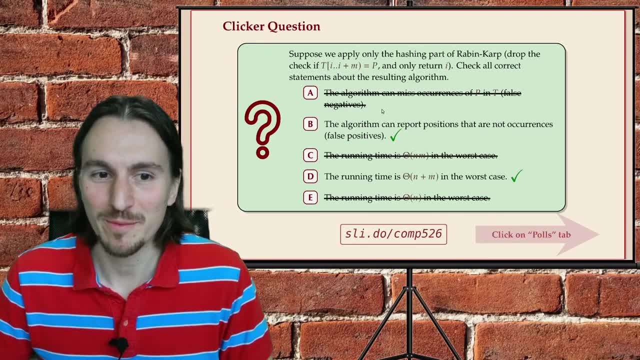 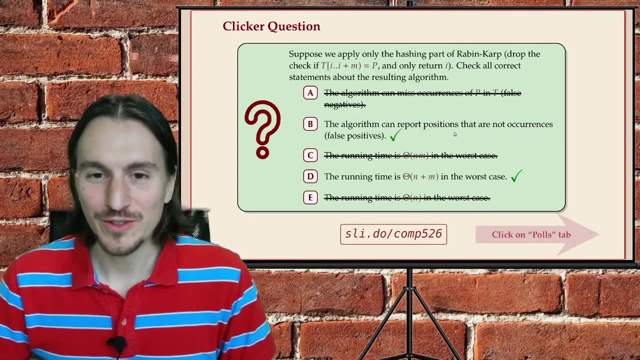 have a different hash for the same string. That cannot possibly happen And you all agree with this, most of you. It can report false positives positions where the hash is the same, but we didn't do the check So we don't know for sure. 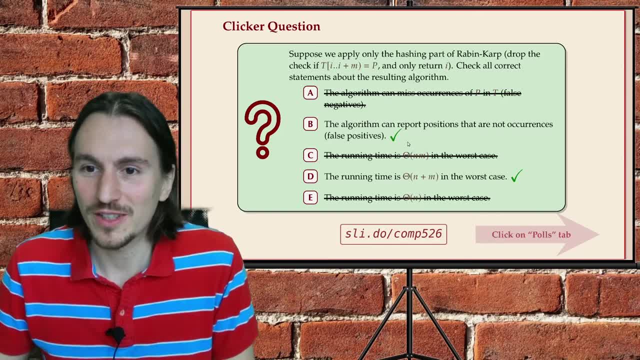 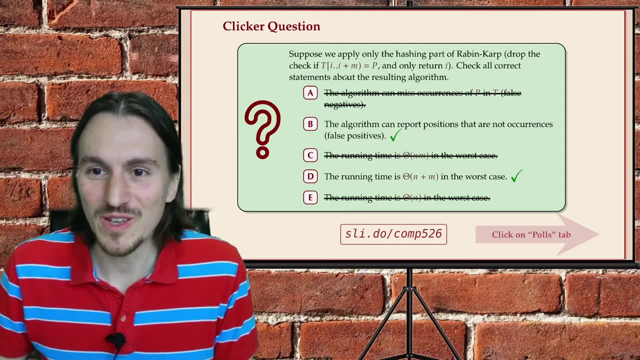 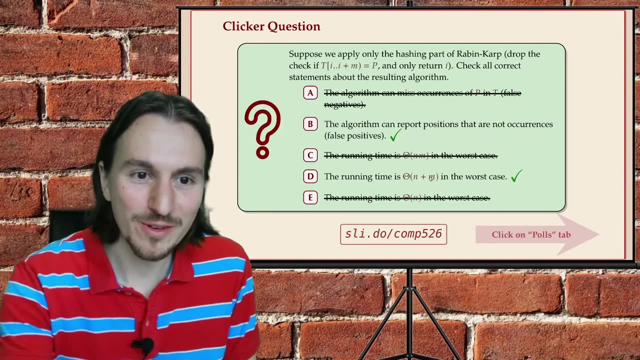 sure, but in some applications maybe this is good enough, depends. the worst case: running time now actually is linear and the reason for that is that we skipped the only thing that was expensive. okay, all the rest is just zoom through the text and do constant time update to the rolling hash. 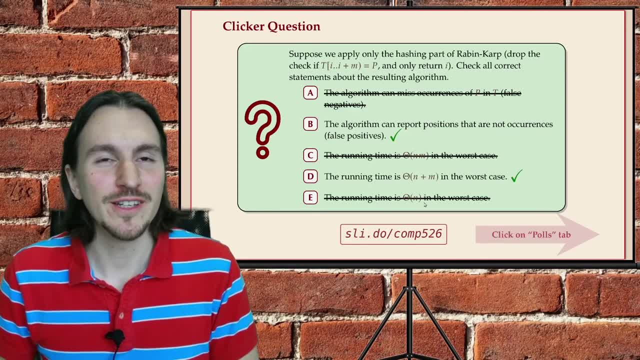 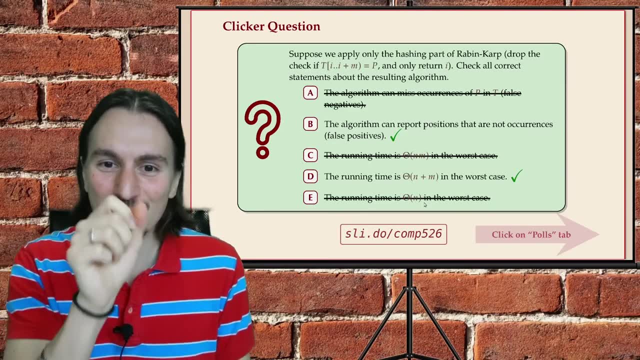 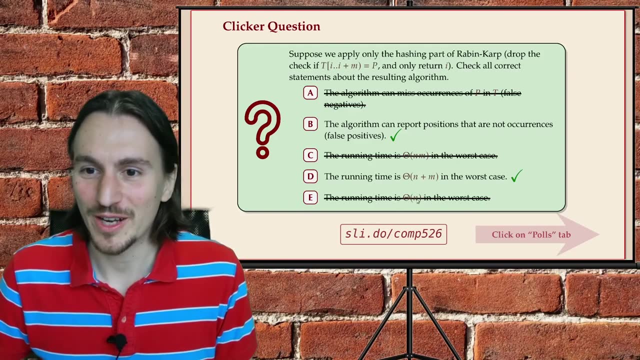 the last statement is not correct because you do have to initialize the first hash. you have to first run through the pattern for the very first beginning. you can do updates in constant time whenever you move through the text after that. but for the first value you need to find the full hash. 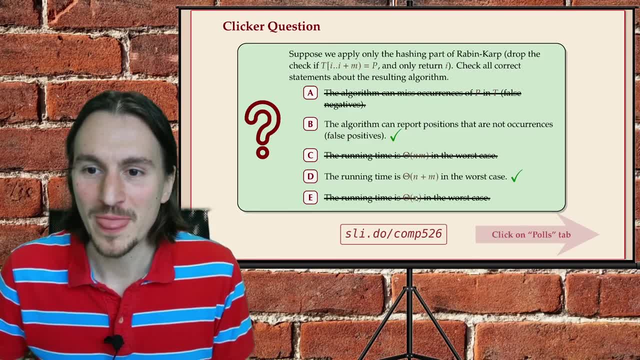 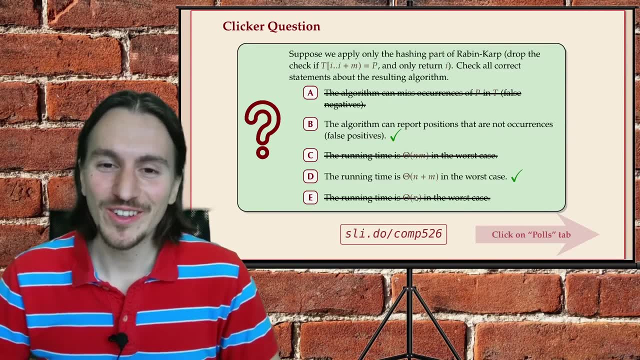 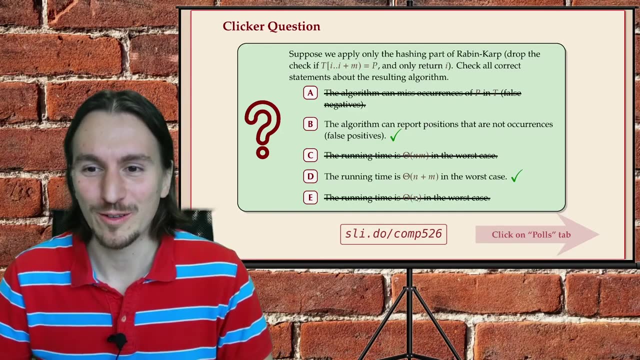 of the pattern and that needs theta m time. and now, in a very stupid scenario, a user might give you a longer pattern than your text is. you could have a separate check to say: hold on, guy, you're man, you're. you're looking for something that's longer than the text. there's no way you can find this. 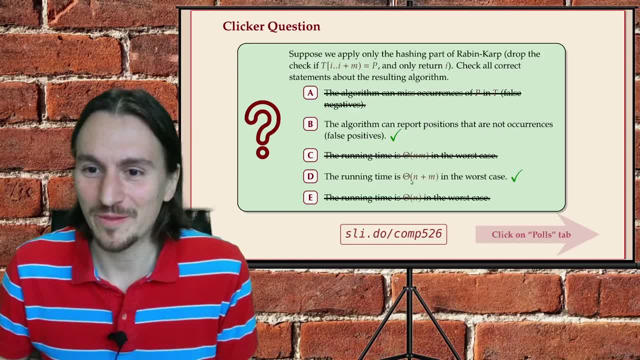 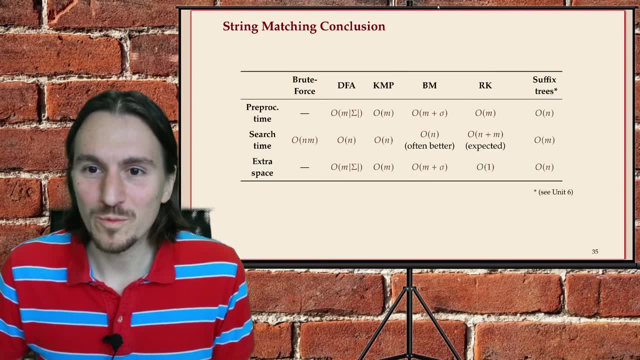 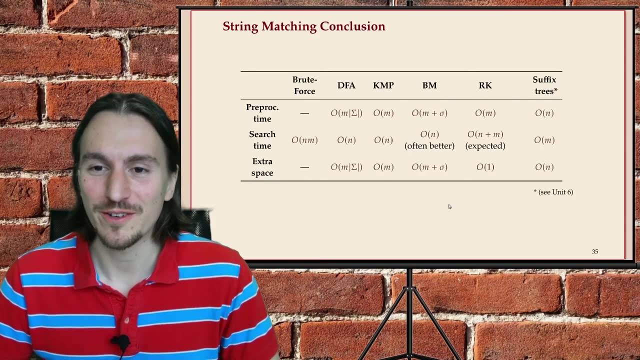 here, but if you're not special casing this, um, your running time would be like this and not that. all right, um. with that, um, we come to the end of unit four on the, the elementary string matching algorithms, uh, and i prepared a nice slide that uh summarizes the different pros and 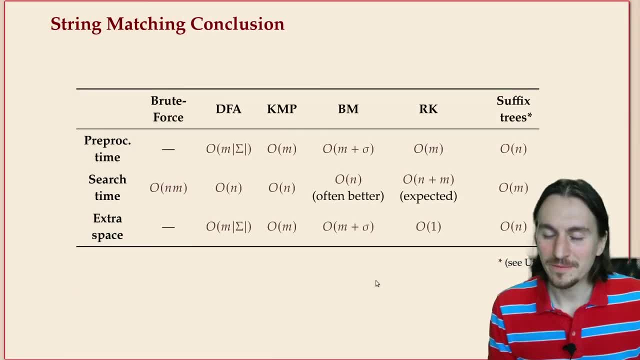 cons of the different methods. um, yeah, that just works if i move a little bit to the right. so, uh, we've seen the brute force method, the finite automata, kmp boy or more rabin carb, and we'll see suffix trees, uh, the week, next week probably, um, and they have. 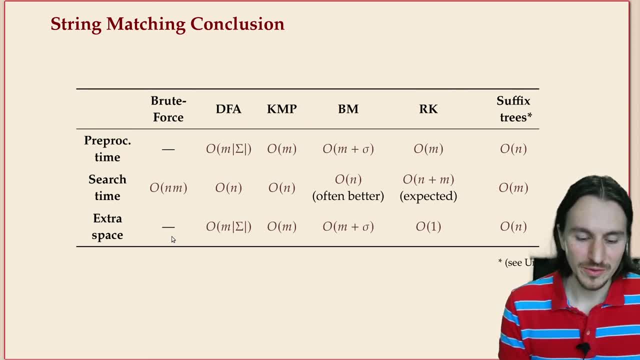 different. they have different um pros and cons. in terms of pre-processing time, uh, brute force doesn't need any here, uh, but the other methods all do some sort of pre-processing to become efficient and, um, here the details really matter. um, i don't know why i didn't put sigma here, so it's the same. 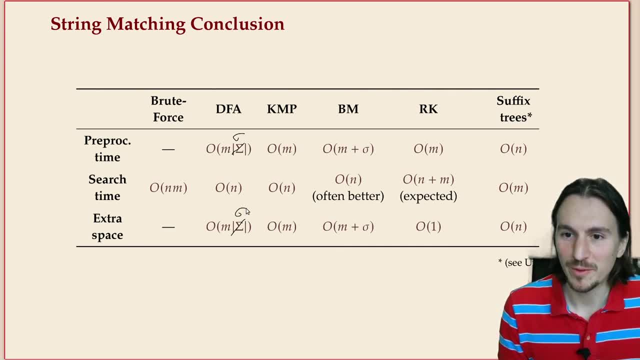 thing. the little sigma is the size of the alphabet and the search time here is given in: uh, the expected or in the typical case, not the worst case. you have to look that up. but this is, this is more of the, the punchline that you usually need: uh, we. you can ignore the last column for now. this is just.